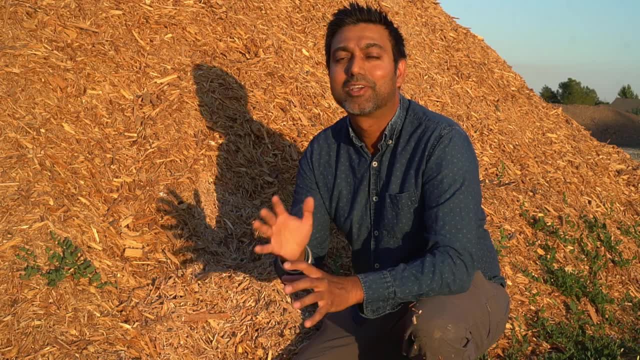 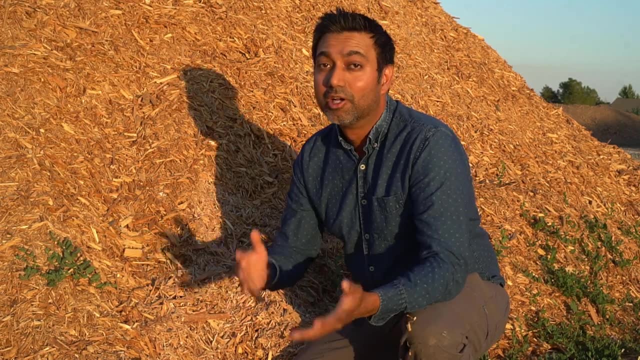 best way to get free wood chips, and i made a separate video on how you can get free wood chips as well. you can also use a service like chip drop. however, in my area they don't actually make it this far, so i have to contact some of my local arborists to get my wood chips. however, 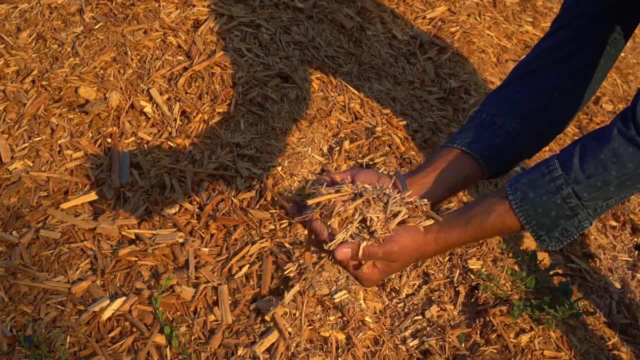 please note, pine needles and wood chips can lock up the nitrogen in your soil, so you don't have to worry about that. you don't have to worry about that. you don't have to worry about that. you want to add wood chips into your soil and plant right away. you want to add wood chips into your? 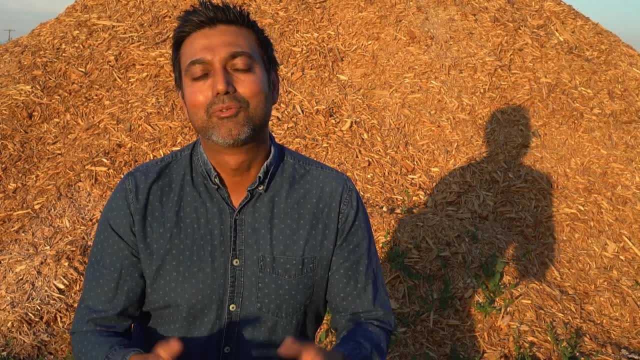 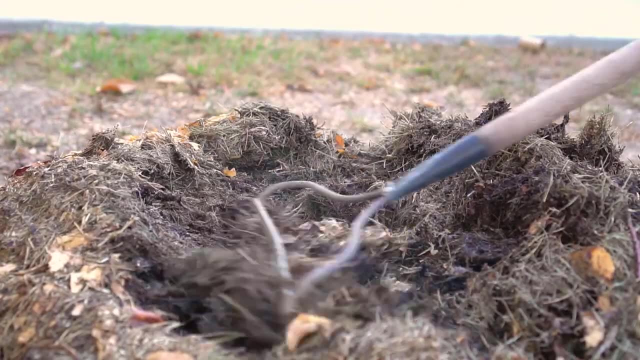 soil at least three to six months before planting, so the wood chips have enough time to decompose, just like compost. need carbon and nitrogen to decompose similarly, which is provide carbon and they look for the microbes. look for the source of nitrogen in your soil to decompose the carbon. 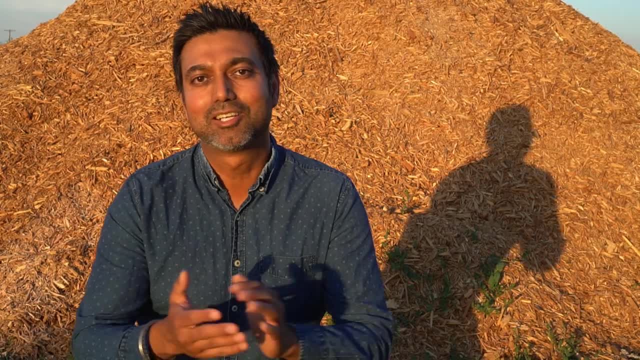 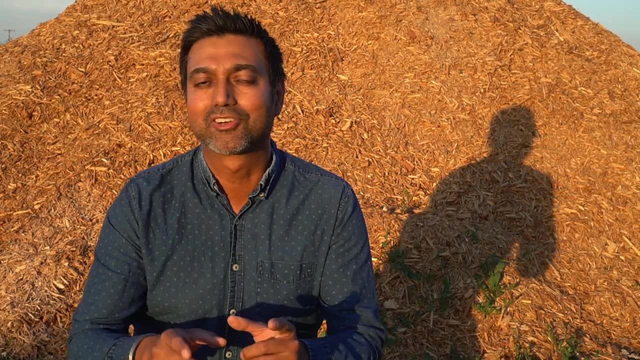 the microorganisms use the carbon and nitrogen in the decomposition process. so you want to make sure the wood chips are already decomposing before planting and you always want to add your fertilizer when you plant, not when you spread wood chips or when you add wood chips into. 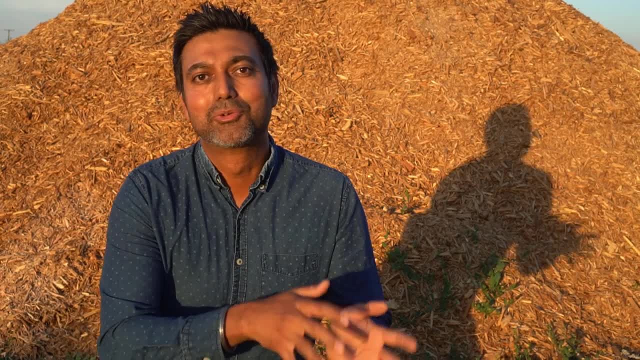 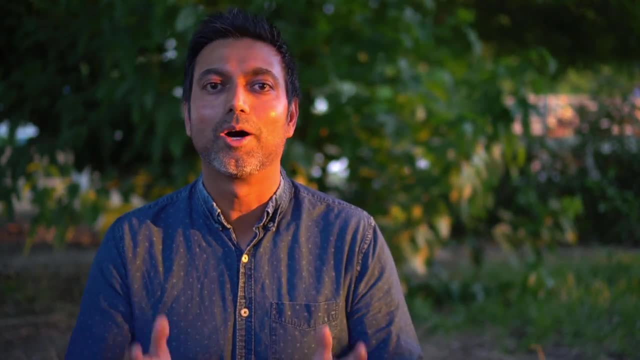 your ground, because all the nitrogen from your fertilizer will be used up to decompose wood chips rather than providing to your plants. most plants like ph between 6.0 and 6.8 to uptake nutrients and do really well. however, certain plants like alkaline soil or others like more acidic soil. so blueberries, bezels and potato. they love acidic soil, while lavender, sweet potatoes and asparagus love alkaline soil. so before you get started, you first must know the current ph level of your soil. let's say your soil is a 6.0, which is a little bit acidic, and you want to grow sweet potatoes or lavender. you must raise the ph level of your soil by at least half a point, or a point to bring it down up to 6.5 or 7.0. however, let's say your soil level, soil ph level is at 6.5 and you want to grow. 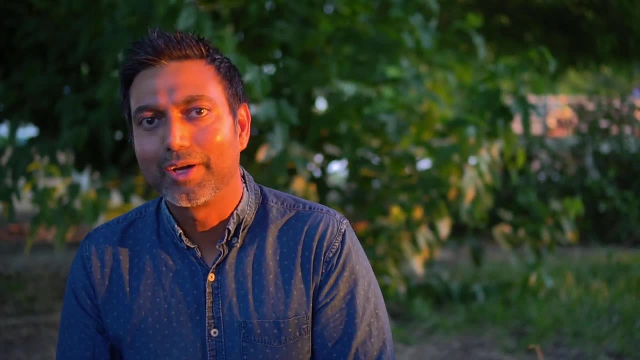 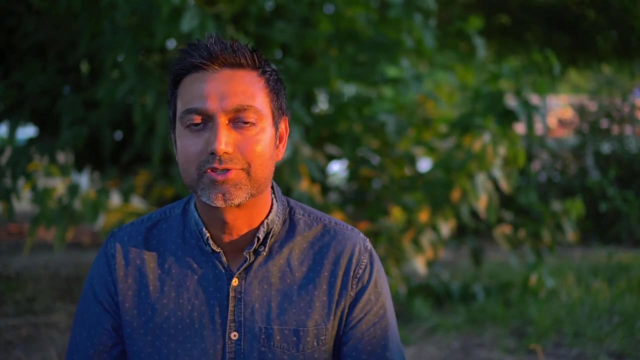 blueberries. you need to bring it down to 4.5 or 5.0 in order to grow blueberries. now here are some things that you can do to know the exact ph level of your soil. you can just use a soil moisture meter that also has a ph level setting to know the ph level of your soil. now that'll give you a rough. 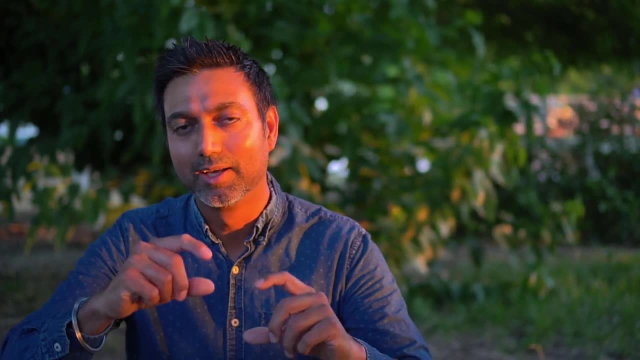 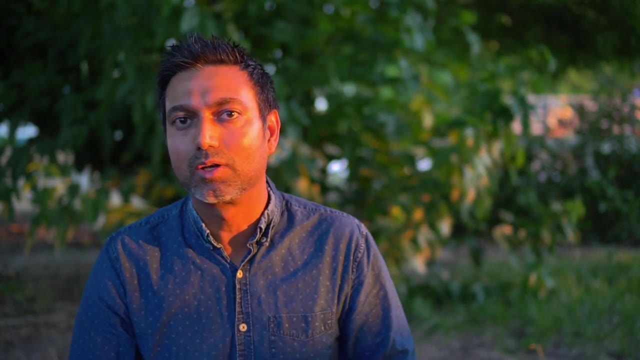 estimate. if you want to know the exact ph level of your soil, you can use soil testing kits to actually know the the actual color change, to actually match up to know the exact ph level of your soil. or you can take a sample of your soil in a quart bag. just use a quart bag or a gallon bag, fill it with soil. 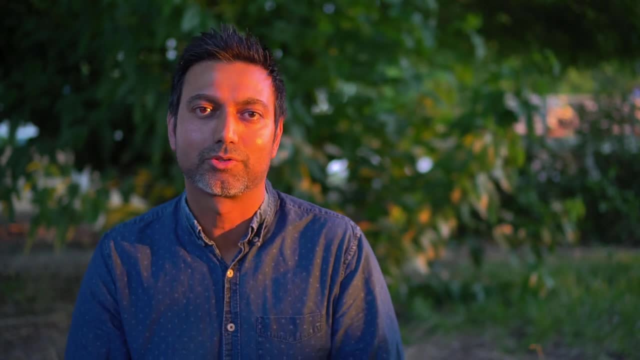 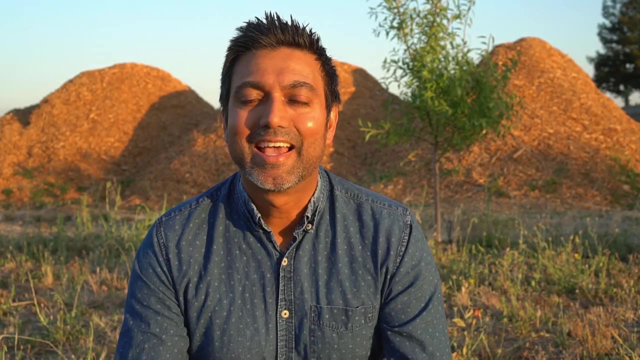 send it to a soil lab in your area and they can do the analysis on your soil and give you a ph level- 30 to 40 dollars. to do one sample analysis, when i prepared my ground to plant blueberries, i added eight truckloads of wood chips into three acres of land to actually acidify the soil. 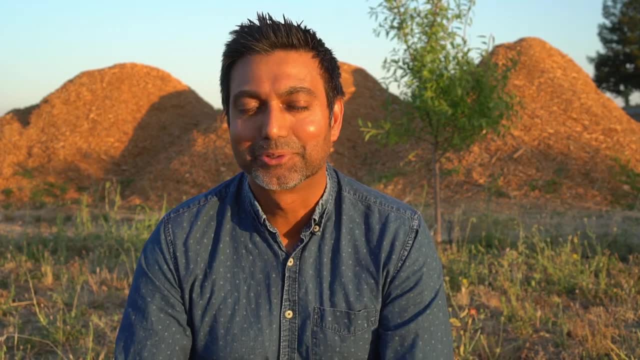 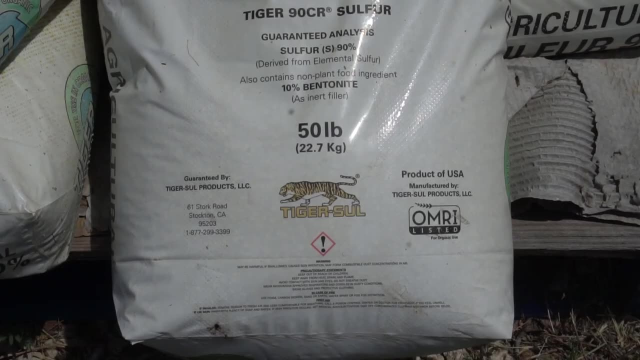 and i use another material, another input material, to lower the ph level of your soil as well. that's coming up next and that's sulfur. i use tiger 90 sulfur. this is approved for organic gardening and it is omri listed. this is how sulfur looks like in bags and to lower. 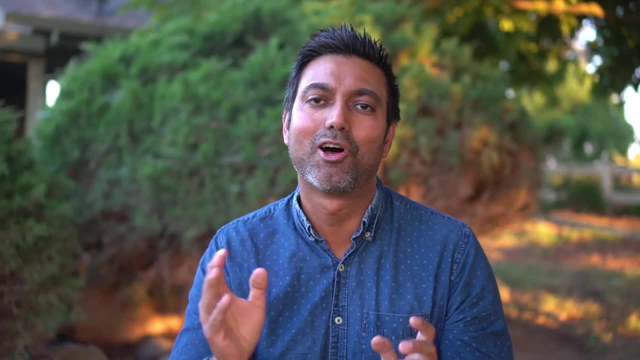 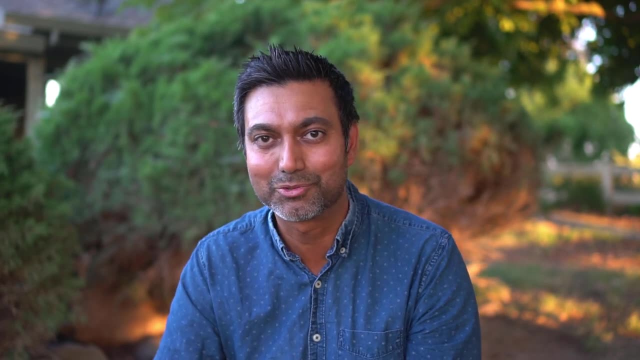 the ph level of your soil. here are the calculations. i know a lot of people asked in the blueberry video on how to lower the ph level of your soil and how much sulfur you need to actually lower the ph level of your soil. so i thought i'll make a totally separate video on how. 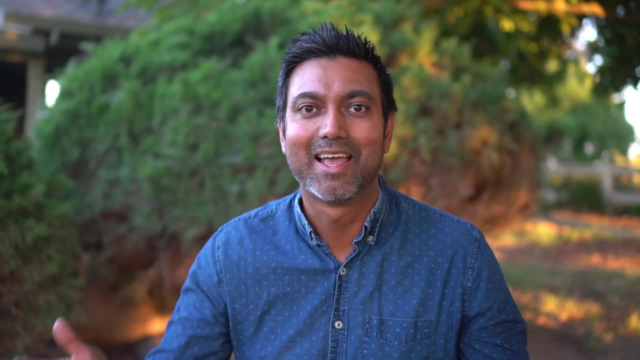 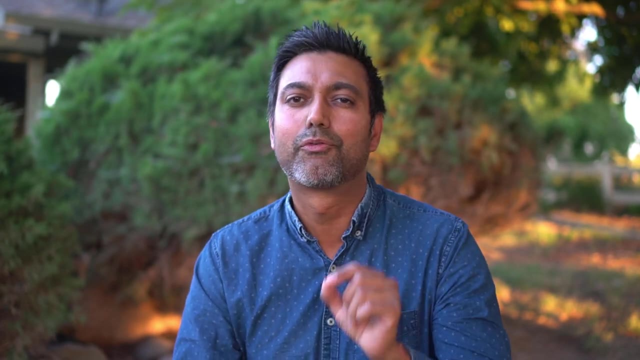 to adjust ph level of your soil, which covers detailed information. and here we are. so take notes, get a paper and a pen, because i'll be giving you some numbers. so to lower the ph level of your soil, you first must know the current ph level of your soil. so let's say your soil is at 6.5. you also must know the type of soil you have. you have sandy soil or clay soil or low me soil. that will play an important role in how much sulfur you need to add. so for sandy soils in 100 square foot area you need one pound of sulfur to lower the ph level by one point. so if 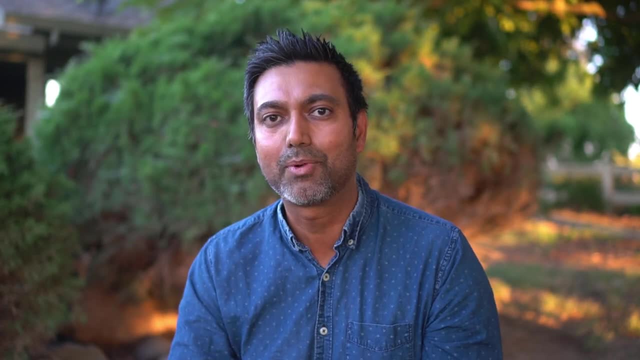 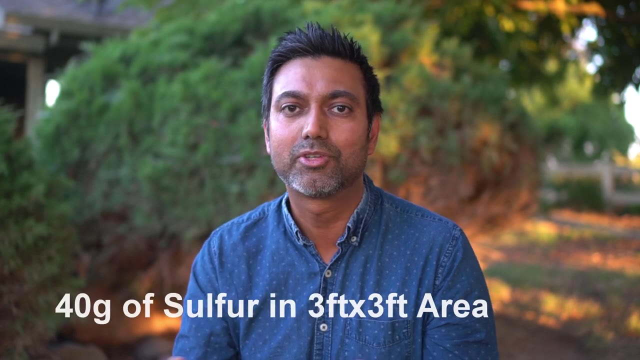 you're 6.5 and you want to lower the ph level to 5.5, you'll sprinkle one pound of sulfur over 100 square foot area. now to give you a context: in a three foot by three foot area, that's about 40. 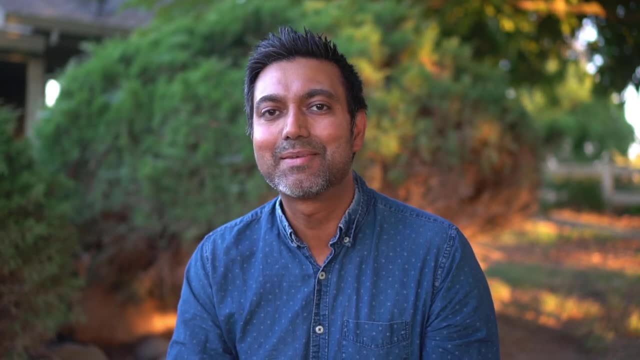 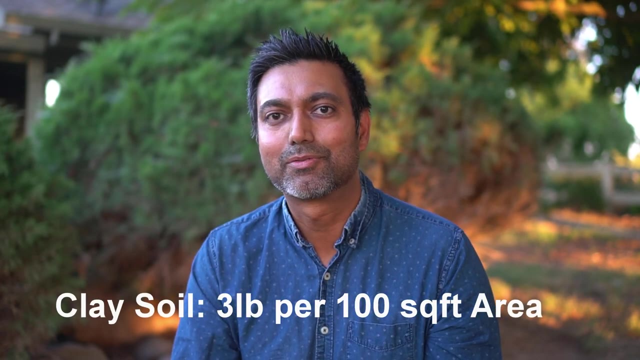 grams of sulfur. now in clay soil you need three times as much sulfur to lower the ph level of your soil. so in the same 100 square foot area you'll need three pounds of sulfur to lower the ph level by one point. so in three feet by three feet area that comes to about 120 grams, which is 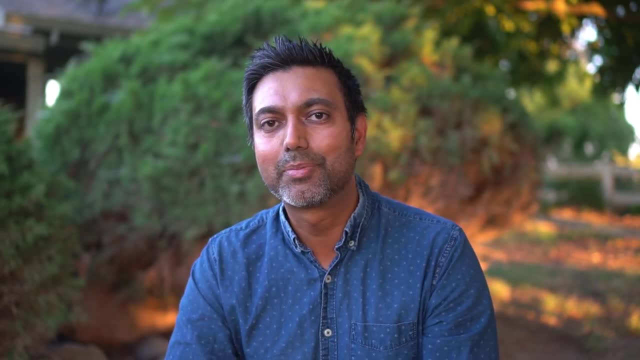 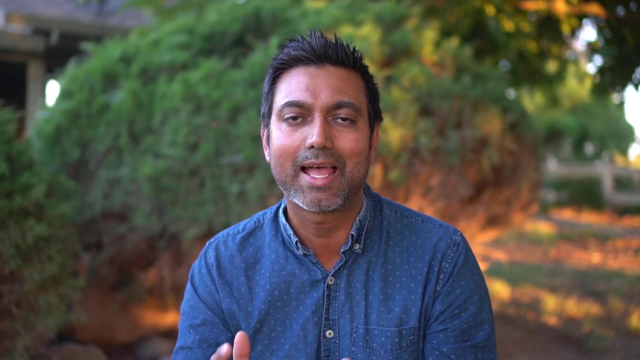 about quarter of a pound. now let's say you want to bring your ph level by two points from 6.5 to 4.5 in clay soil, so you'll need 240 grams of sulfur, which is about half a pound in three foot by three. foot area. now let me throw a little bit more numbers at you to wrap your head around it now. let's say you want to bring the ph level down to 5.5. from 6.5 to 4.5 in clay soil in a row. that's three foot wide and 100 feet long. that's 300. square feet. now we already know that every hundred square foot area in sandy soil you need one pound of sulfur. in clay soil you need three pounds of sulfur. now we have 300 square feet, so we gotta multiply three by three. that's nine pounds of sulfur to bring the ph level by one point. now we gotta bring the ph by two points from 6.5 to 4.5. so you'll need 18 pounds of sulfur to do the same. when we planted blueberries in three acres, we ended up using two tons of sulfur, which is about four thousand pounds of sulfur. now you want to add sulfur- at least six. 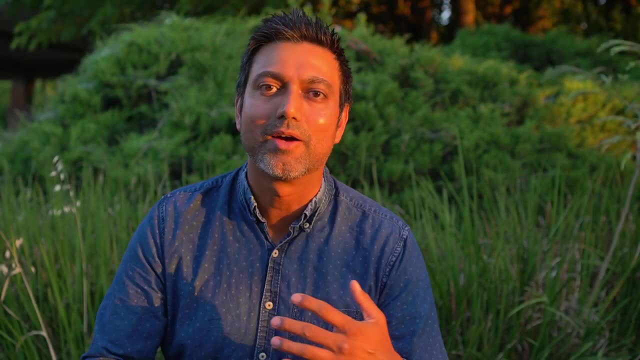 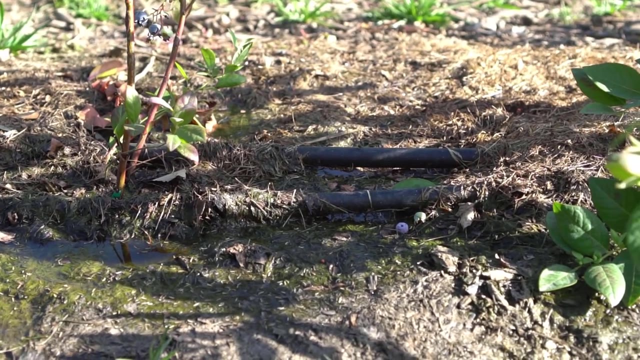 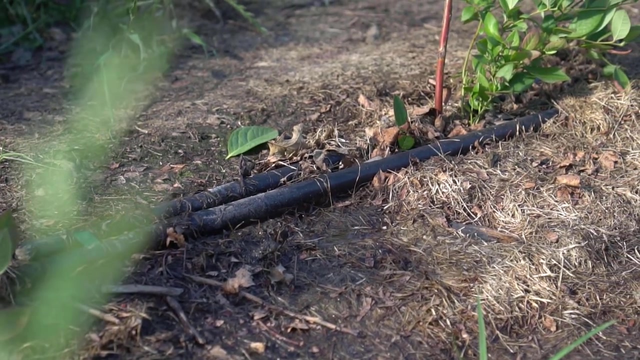 months before you plant as well, because sulfur takes time to have a reaction process in the soil to start lowering the ph level of your soil. now you also must know the ph level of your water. so if you keep watering the plants or your soil with 7.0 water over time, the soil ph level will 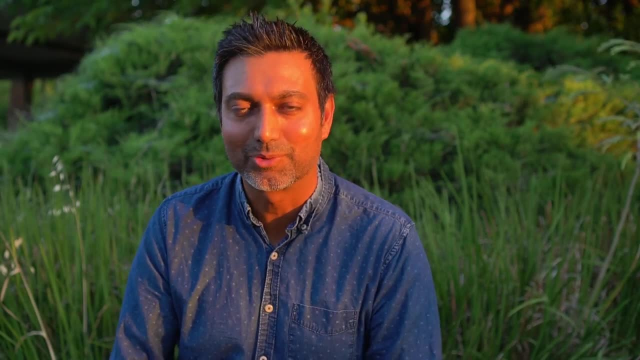 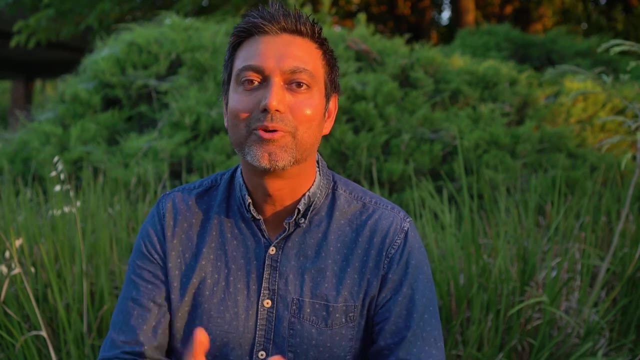 rise and you need to apply something to lower the ph level of your soil as well. so another thing you can use in home gardening or in your backyard to lower the ph level of your soil: you can use just plain old vinegar. use a cup of vinegar to a gallon of water, which is about 3.75 liters of water. 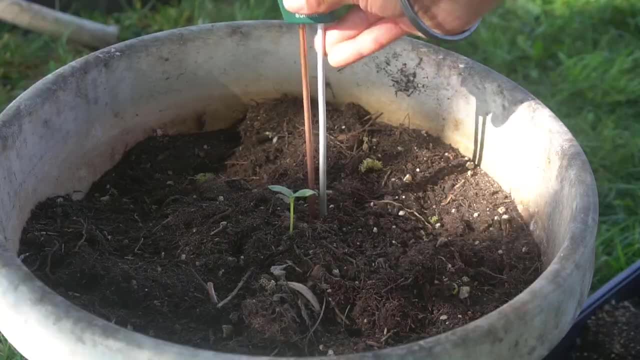 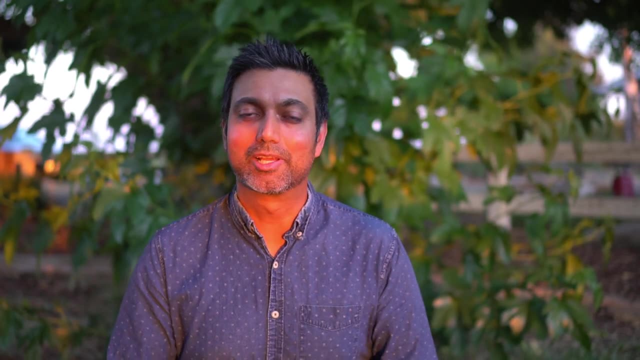 water your plants with this solution once a week and keep checking the ph level of your soil. once you reach the desired ph level, you can stop using vinegar. now let's talk about raising the ph level of your soil, and for that you need lime, which is calcium carbonate. 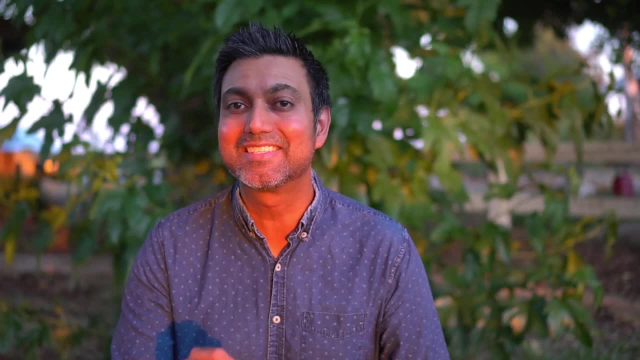 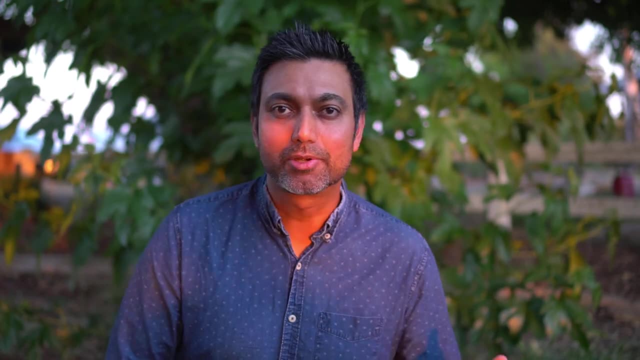 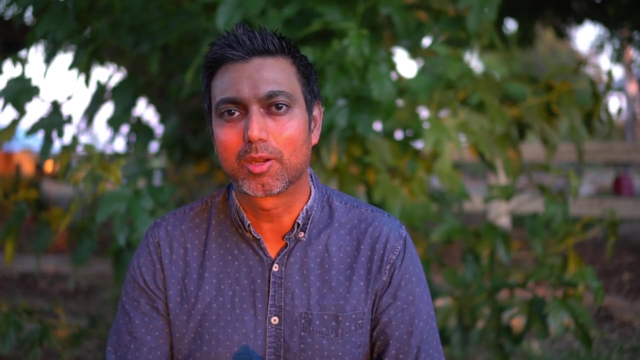 and you want to pay attention to one particular number, which is the cce number, which is calcium carbonate equivalent number. now, some calcium carbonate or lime is sold at 90 or 100 percent. you need 100. if you use 100, you'll need about 1.2 pounds of calcium carbonate or lime per 100. square foot of area. so you'll use the same calculations that i gave you before for sulfur, but tweak them to use 1.2 pounds for 100 square feet instead of just one pound. now, if you use 90 cce, you need about 1.3 to 1.4 pounds of calcium carbonate for 100 square foot area. 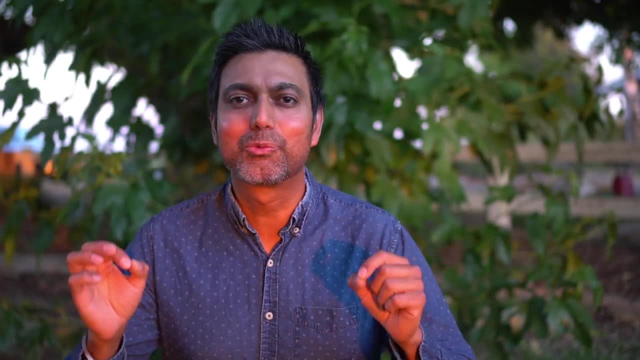 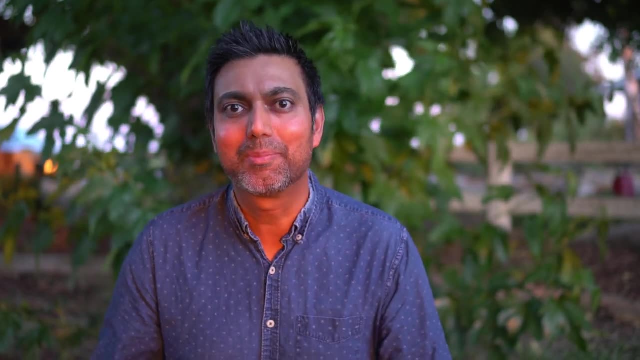 you can also use wood ash or potash, which is also a really good source to actually raise the ph level of your soil and make yourself alkaline, and also to add potassium and calcium into your soil. they are rich in potassium and calcium, so i always save all of the ash from our 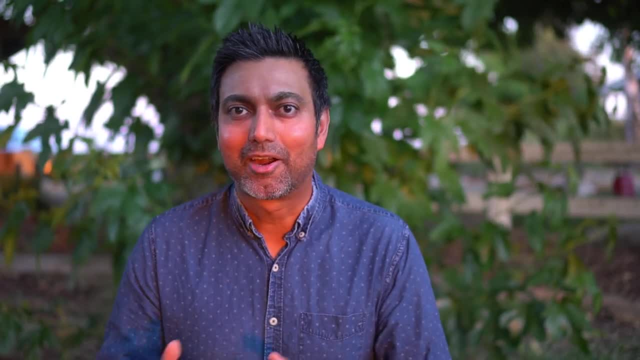 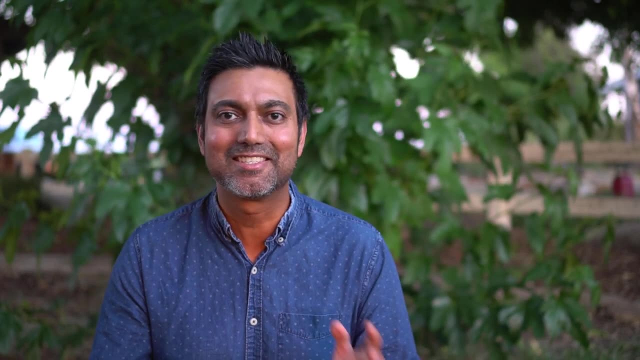 fire pits from our fireplace and i use them in garden when i grow sweet potatoes, when i grow lavender and i grow other plants that love alkaline soil. now you also want to pay attention to the cce number for wood ash. now, the cce number for wood ash depends on how condensed the wood. 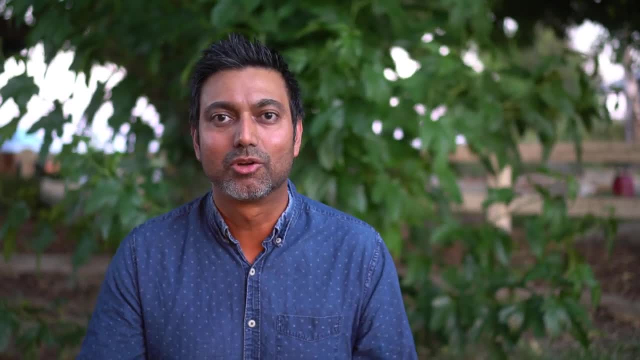 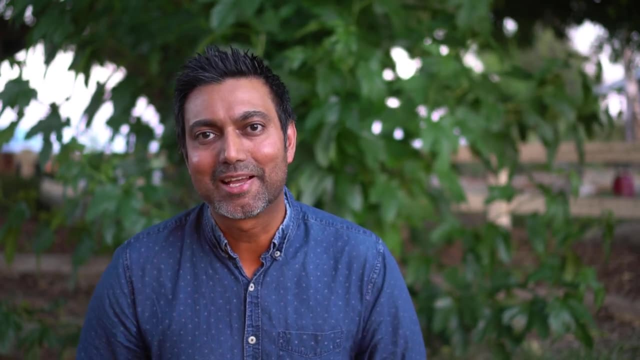 ashes and it varies from 25 percent to 50 percent. so depending on how condensed your wood ash is that you get from your fireplace or your or your fire pit, you'll use two to four times as much wood ash as compared to lime. i hope all of this information is very useful for you to either.